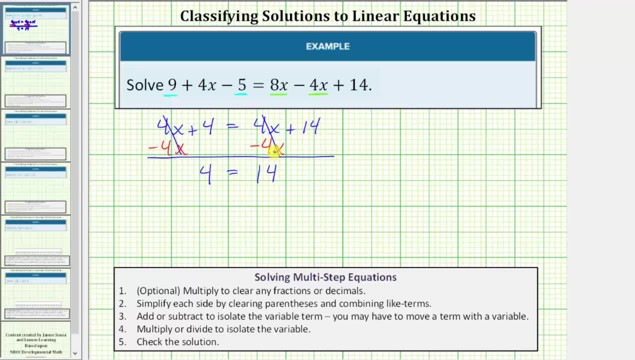 The right side simplifies to 14.. So notice, in the process of isolating the variable, the variable terms simplify out and we're left with the equation four equals 14.. Well, we know, four equals 14 is false. So, because this equation is false, 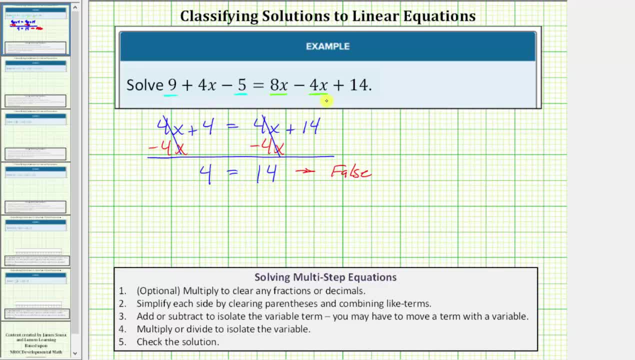 that means there are no solutions to the original linear equation. So we can say the equation has no solutions. Again, in the process of solving the equation, the variable terms simplify out and the resulting equation is false. this indicates the equation has no solutions. 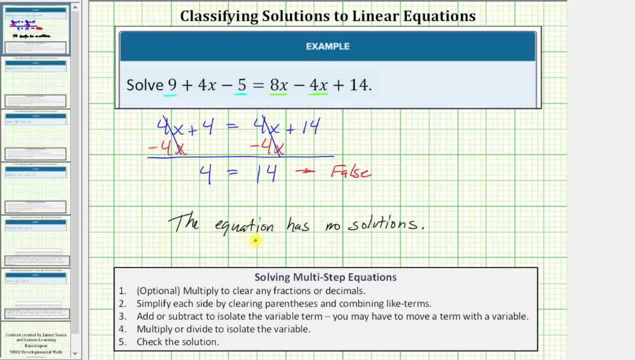 And sometimes we say the solution does not exist, or DNE for short, DNE for does not exist. Let's look at a second example. We have the same type of equation, so for the first step we'll simplify both sides of the equation. 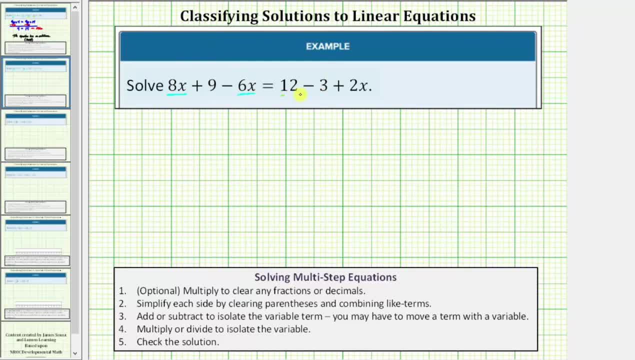 On the left we have two x terms, on the right we have two constant terms. So the left side, eight x minus six x is two x. the left side simplifies to two x plus nine. On the right side, 12 minus three is equal to nine. 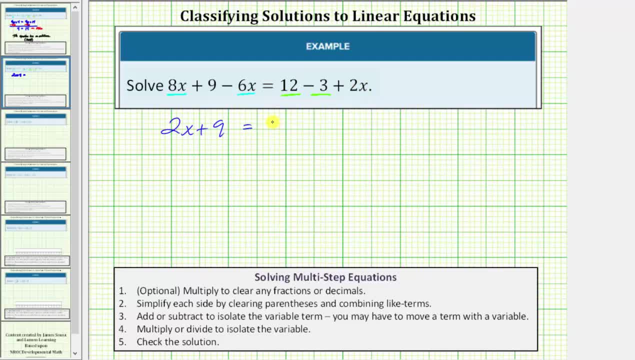 the right side simplifies to: nine plus two x, or, if we want, two x plus nine. Now, looking at the equation closely, notice how the expression on the left is exactly the same as the expression on the right, which means this is going to be true for any value of x. 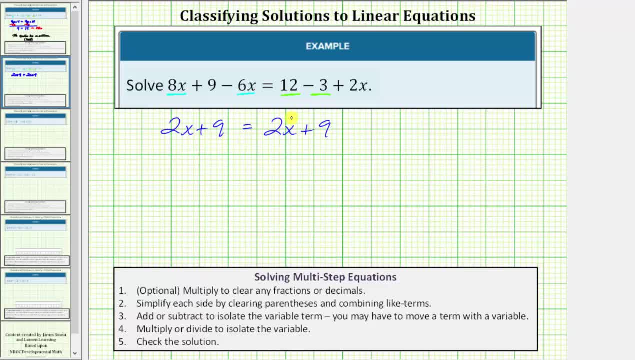 and therefore there's an infinite number of solutions. But if we don't recognize this, the next step would be to add or subtract, to isolate the variable term. So to undo the positive two x on the right side, we would subtract two x on both sides. 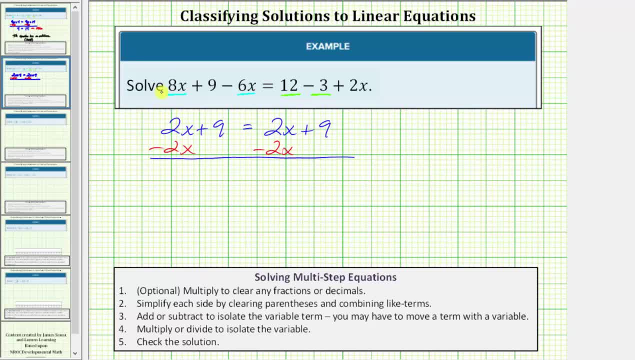 And now we'll simplify. On the left, two x minus two x is zero. the left side simplifies to nine, so we have nine equals on the right: two x minus two x is also zero. notice how the right side also simplifies to nine.